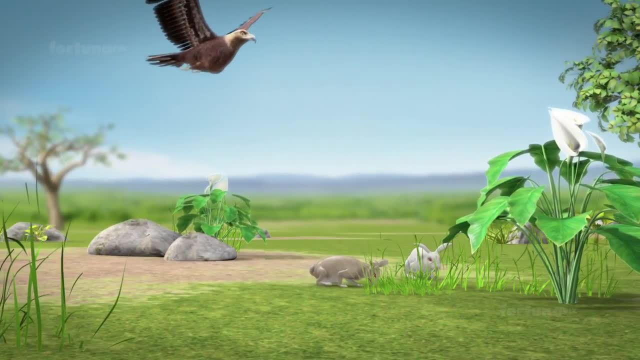 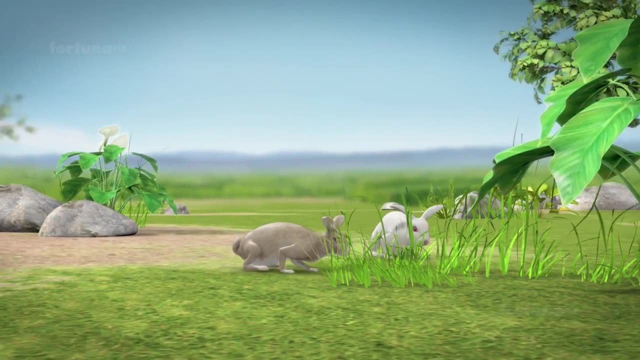 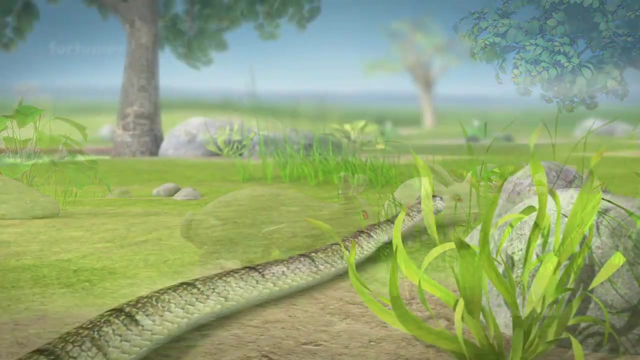 As energy is transferred from one trophic level within the ecosystem to the next, from producers to primary consumers, about 90% of it will be lost as heat as a byproduct of respiration, Similarly as the remaining energy flows into the next trophic level, 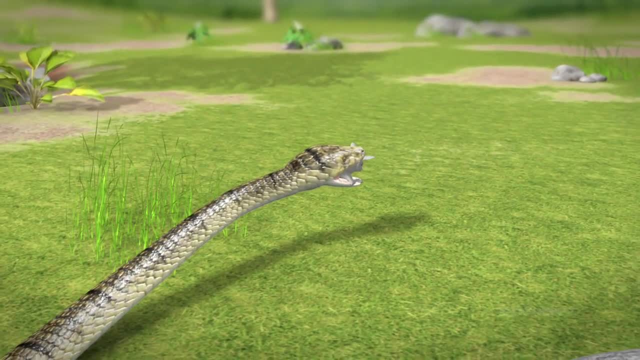 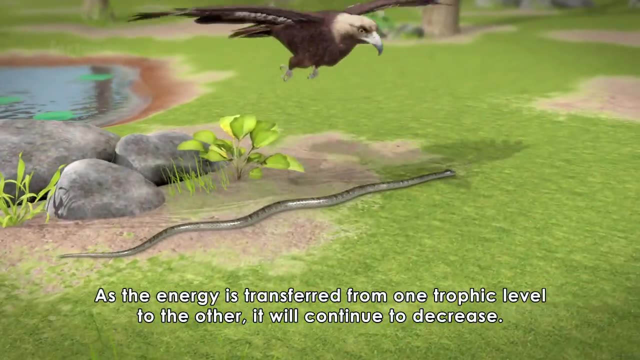 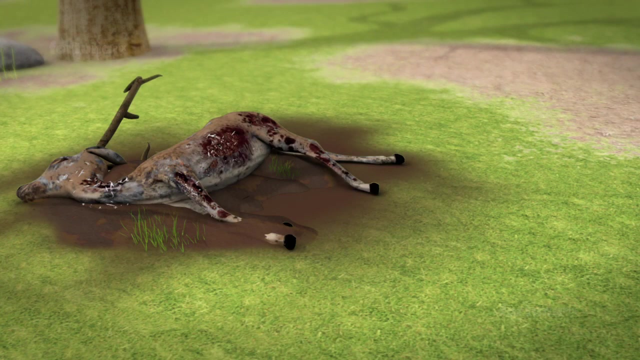 which will be the secondary consumers. another 90% of the remaining energy will be lost as heat. As the energy is transferred from one trophic level to the other, it will continue to decrease Decomposers such as bacteria and fungi. 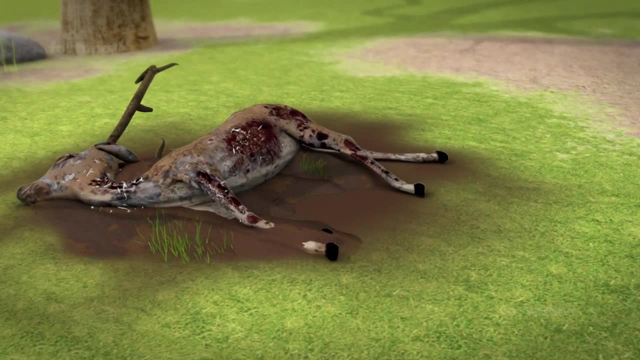 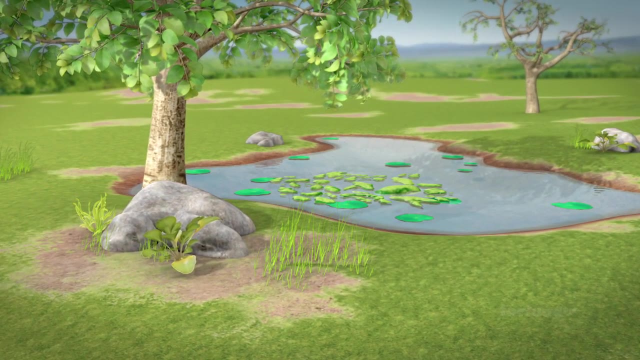 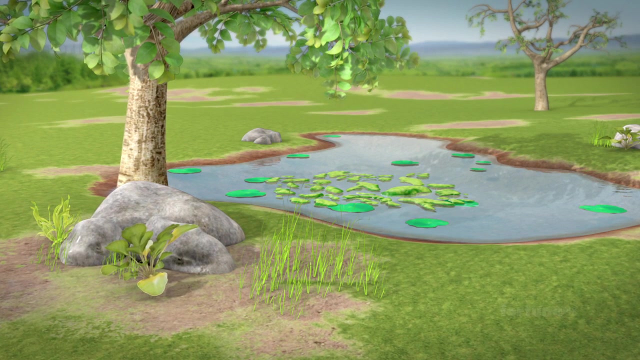 break down dead materials into inorganic substances and produce heat as a byproduct. To better understand how this loss of energy works, let's take a brief look at a simple ecosystem. Suppose grass produces and has 1,000 kilocalories of energy. 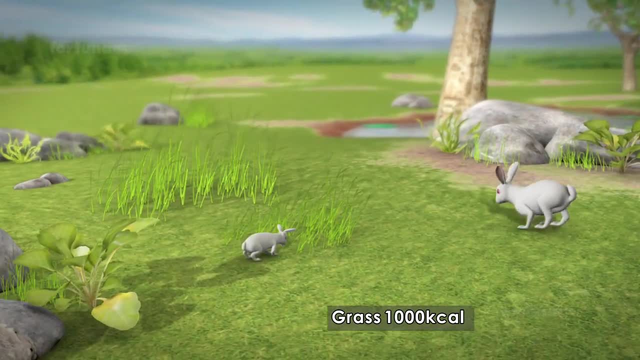 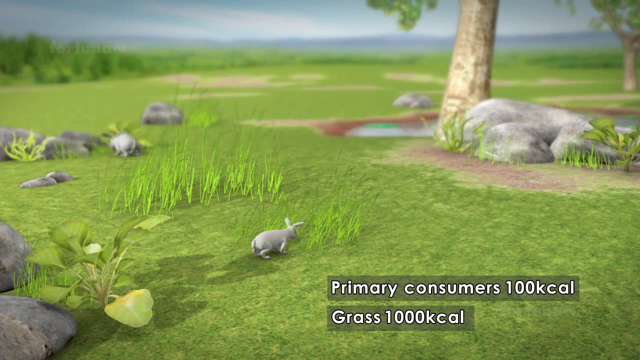 At the herbivore level, the grass will be eaten by mice or rabbits. Primary consumers have an intake of approximately 100 kilocalories. At the next trophic level, mice and rabbits will be eaten by a snake. The secondary consumers have an intake of approximately 10 kilocalories. 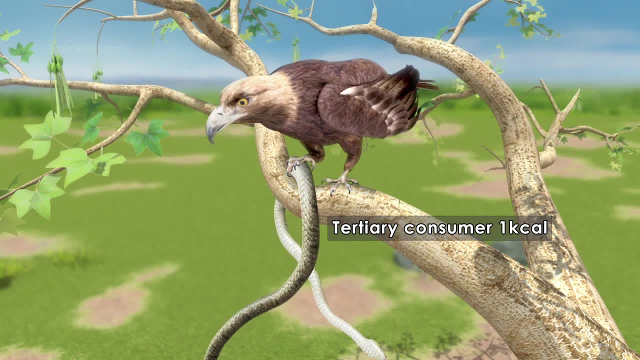 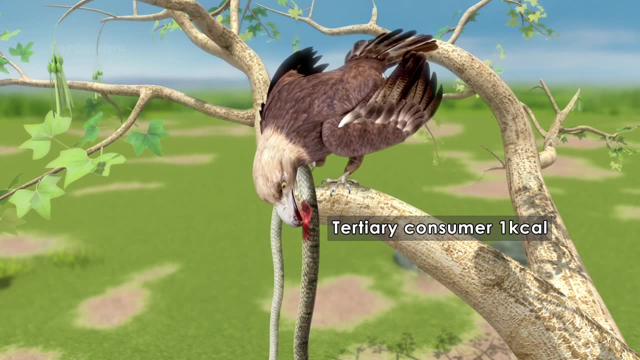 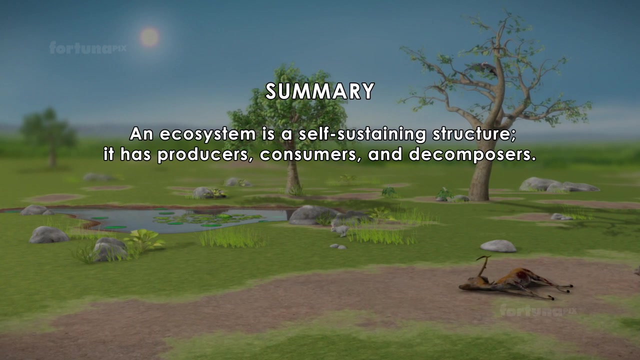 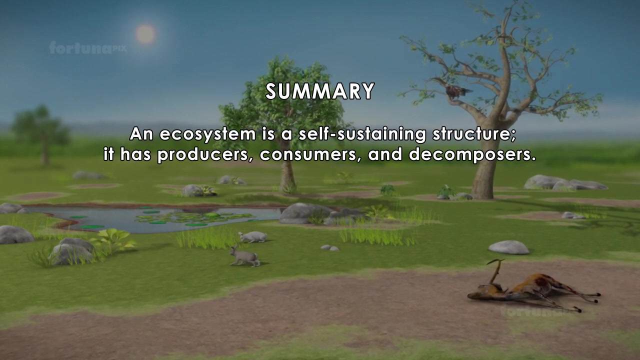 Tertiary consumers, such as eagle, will eat the snake. These consumers will have an intake of only 1 kilocalories. Summary: An ecosystem is a self-sustaining structure. It has producers, consumers and decomposers. The energy from the sun enters the ecosystem by way of producers. 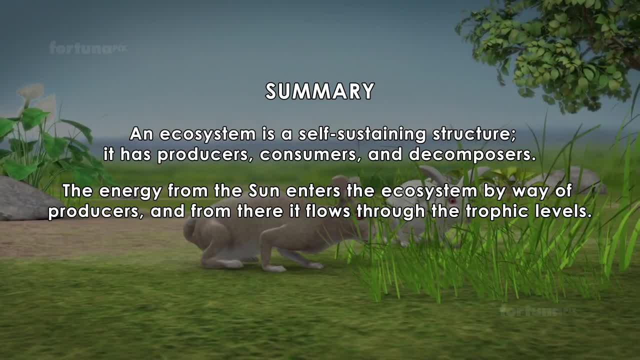 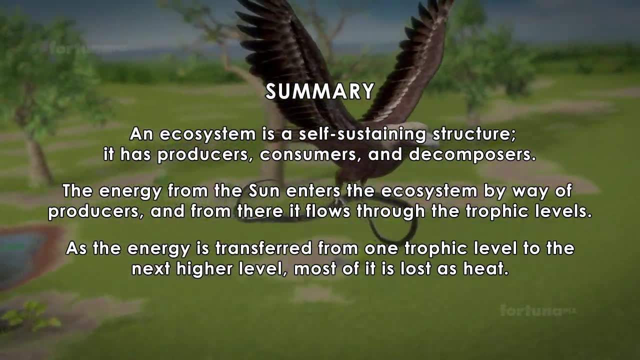 and from there it flows through the trophic levels. As the energy is transferred from one trophic level to the next higher level, most of it is lost as heat.